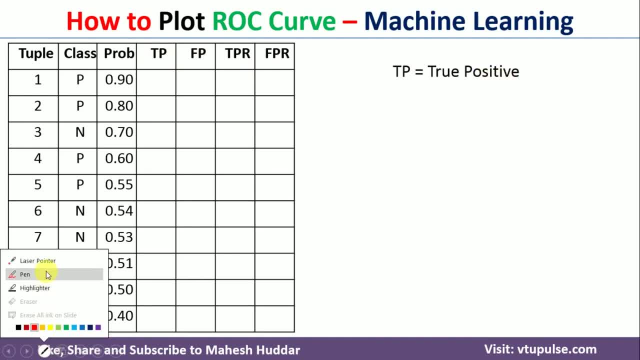 what is TP? TP is nothing but true positive. in this case, What is true positive? Let us assume that the actual class is positive and it is classified as positive. That is nothing but a true positive over here. The second one is false positive. 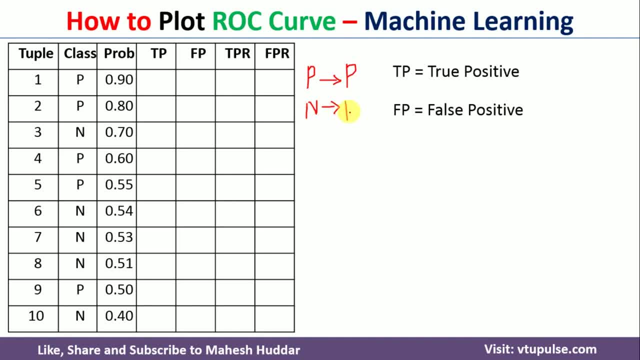 That is nothing. but the actual class is negative. but it is classified as positive. That is nothing but a false positive over here. Once you know these two parameters, you can easily calculate TPR. That is: TPR is equal to TP divided by P. That is TP. we have already calculated. 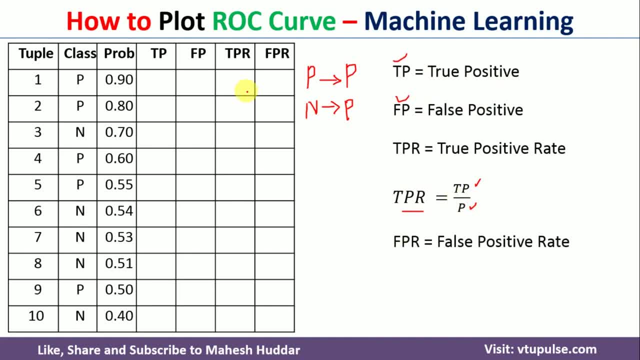 That is true. positive, And P is the number of positive examples. To calculate FPR. we consider FPR is nothing but false positive rate, which is equal to FP divided by N, where N is the number of negative examples. here Now we try to calculate these values. To calculate: 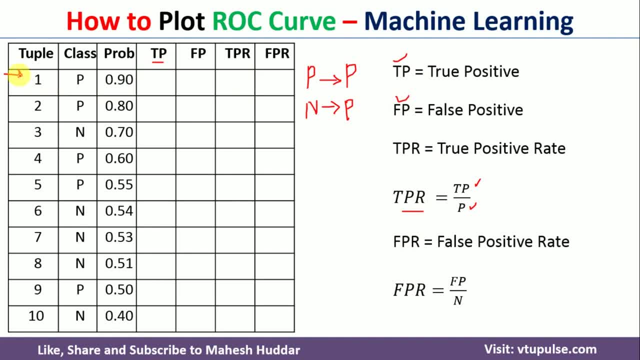 this particular TP, we consider this particular first tuple. here The first tuple's probability is 0.90.. Now we consider this one as a threshold for time being, And if the calculated probability is 0.90 or more, then the tuple is classified as positive here. 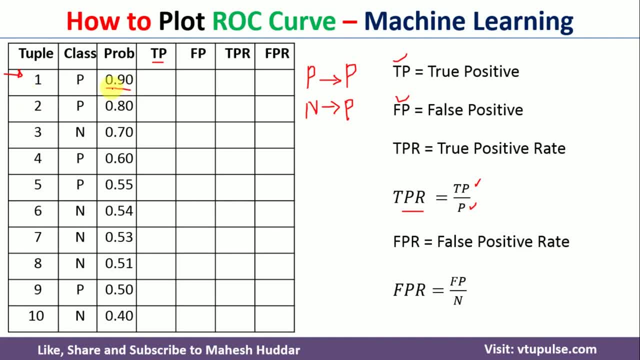 So because this is the only tuple having the probability is 0.90,, this will be classified as positive. here Now the example is positive and it is classified as positive. The meaning is it is a true positive. So we will write one here and false positive will become zero. 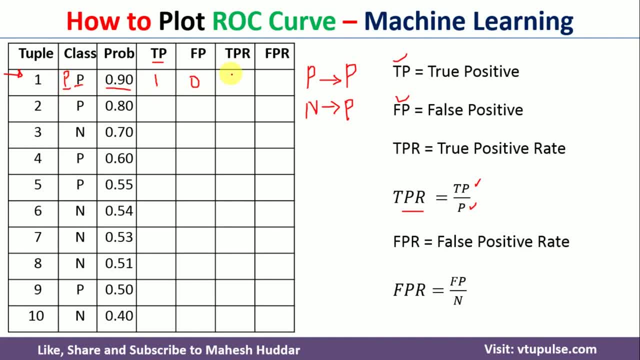 in this case, And the TPR is equal to 1 divided by 5 and FPR is equal to 0 divided by 5.. That is equal to 0.2 here and 0 over here. Now coming back to the next tuple, Once you have, 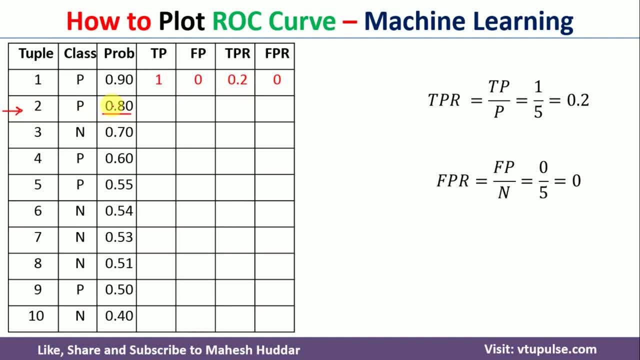 considered the next tuple, the probability is 0.80.. So this will be considered at the threshold here. Now, if the threshold probability is 0.80 or more, the example will be classified as positive. Again, this will be classified as positive and example is actually positive. 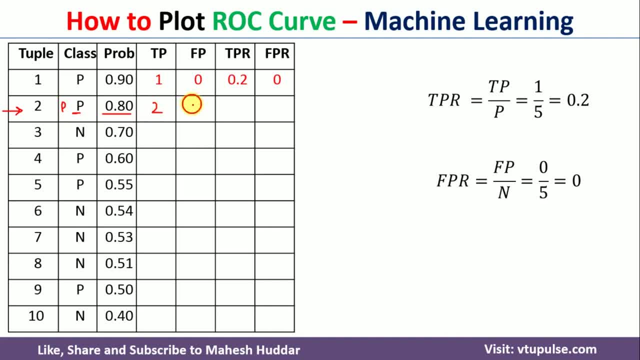 The meaning is true. positive will be incremented by 1, that will become 2 and FPR will remain zero. here And then we need to calculate TPR. TPR is equal to 2 by 5 and FPR is equal to 0 by 5.. 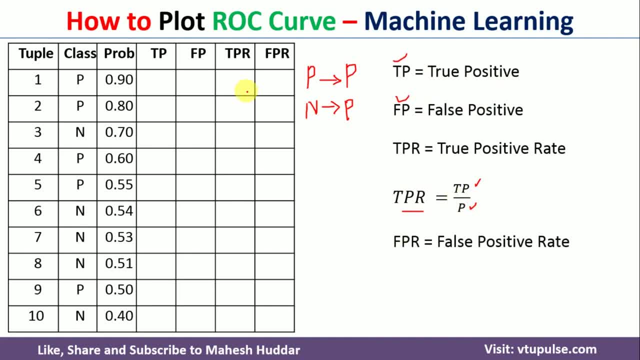 That is true. positive, And P is the number of positive examples. To calculate FPR. we consider FPR is nothing but false positive rate, which is equal to FP divided by N, where N is the number of negative examples. here Now we try to calculate these values. To calculate: 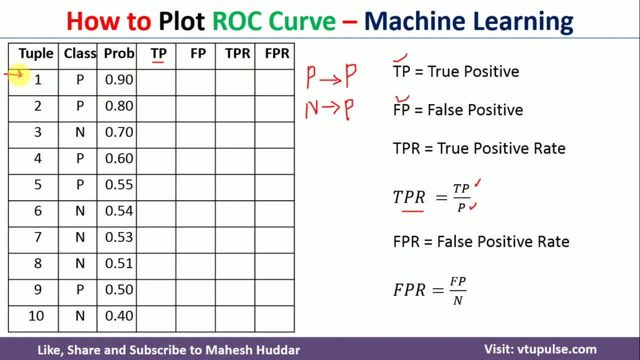 this particular TP, we consider this particular first tuple. here The first tuple's probability is 0.90.. Now we consider this one as a threshold for time being, And if the calculated probability is 0.90 or more, then the tuple is classified as positive here. 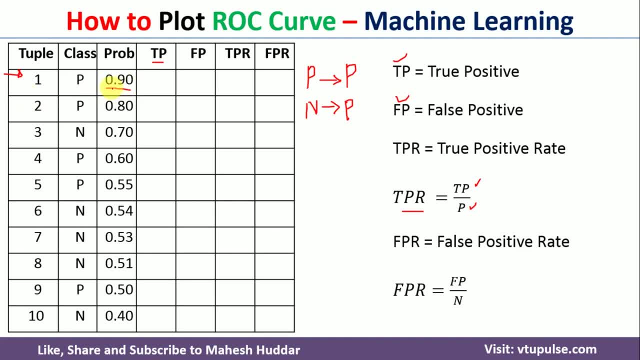 So because this is the only tuple having the probability is 0.90,, this will be classified as positive. here Now the example is positive and it is classified as positive. The meaning is it is a true positive. So we will write 1 here and false positive will become 0 in. 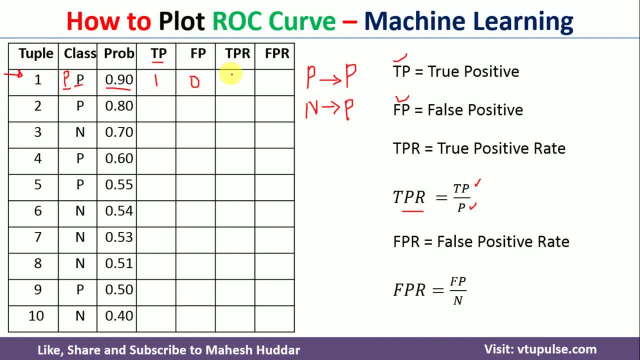 this case, And TPR is equal to 1 divided by 5 and FPR is equal to 0 divided by 5.. That is equal to 0.2 here and 0 over here. Now coming back to the next tuple, Once we have. 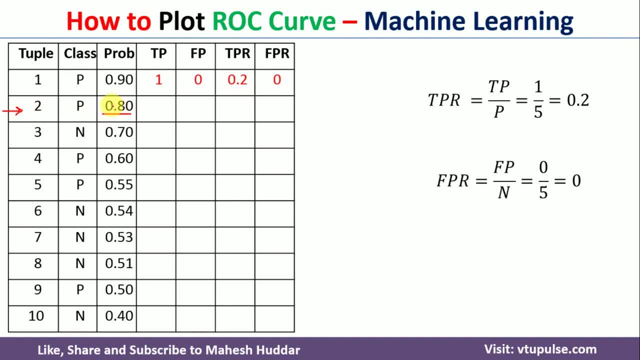 considered the next tuple, the probability is 0.80.. So this will be considered as a threshold here. Now, if the threshold probability is 0.80 or more, the example will be classified as positive. Again, this will be classified as positive and example is actually positive. 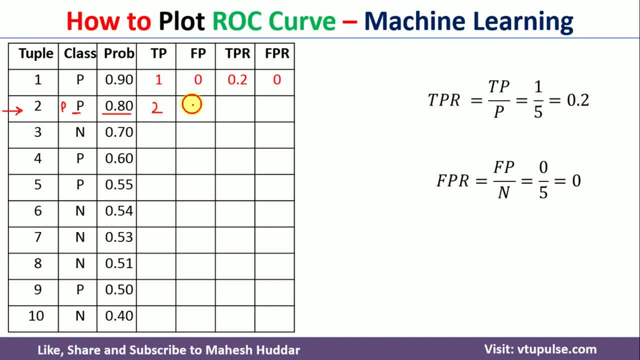 The meaning is true. positive will be incremented by 1, that will become 2 and FP will remain 0. here And then we need to calculate TPR. TPR is equal to 2 by 5 and FPR is equal to 0 by 5.. 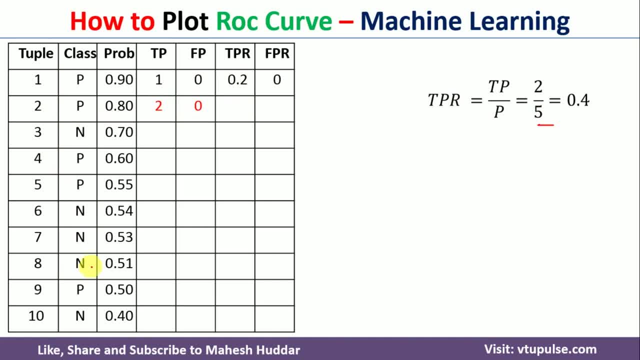 Why? Because there are 5 positive examples and 5 negative examples are there here. So the value is 0.4 and 0 in this case. Similarly, we will consider one more example here. In this case, 0.70 is the probability, So anything equal to 0.70 or more than 0.70 will be classified. 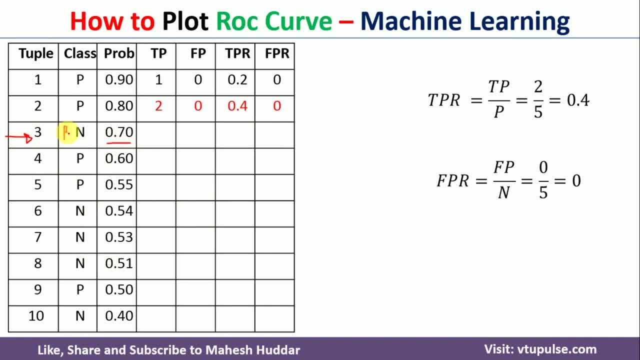 as positive here. So this is again classified as positive. but actual class is what? Negative here? Because of this, it will be considered as a false positive. So false positive will be incremented by 1.. Now it will become 1 here and it will be kept as it is. that is 2 and 1 here And then. 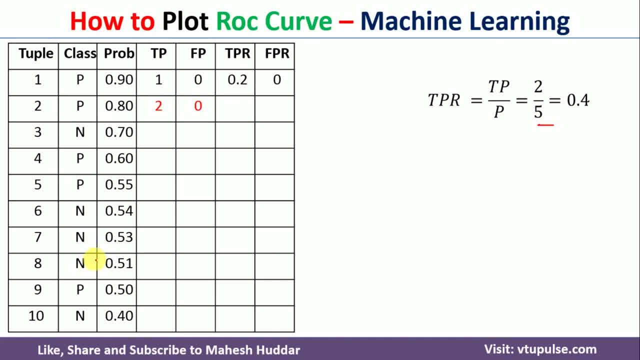 So these are five positive examples and five negative examples are there here. So the value is 0.4 and zero in this case. Similarly, we will consider one more example here. In this case, 0.70 is the probability, So anything equal to 0.70 or more than 0.70 will be classified. 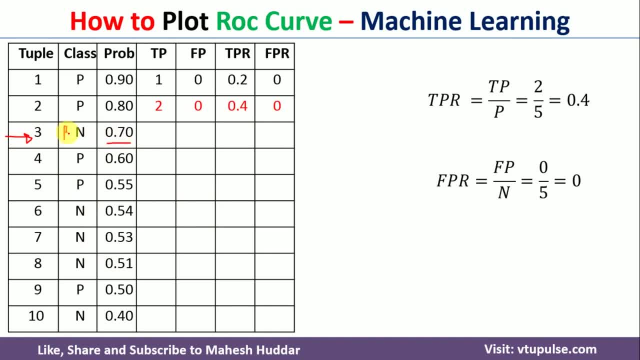 as positive here. So this is again classified as positive. but actual class is what negative here? because of this, it will be considered as a false positive. So false positive will be incremented by 1.. Now it will become 1 here and it will be kept as it is. that is 2 and 1 here And then. 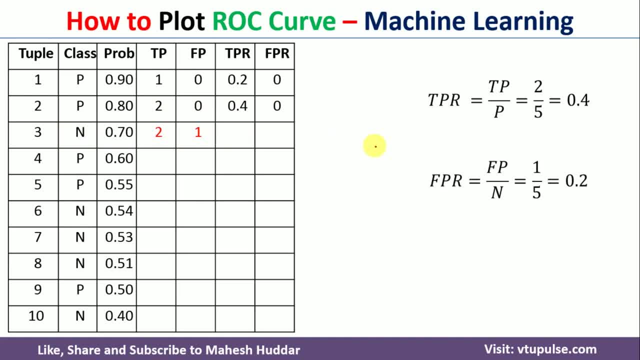 TPR is equal to 2 by 5 and FPR is equal to 1 by 5.. It will become 0.4 and 0.2 here. Similarly, we have to calculate all other- the TPR and FPR- Once you calculate this particular TPR. 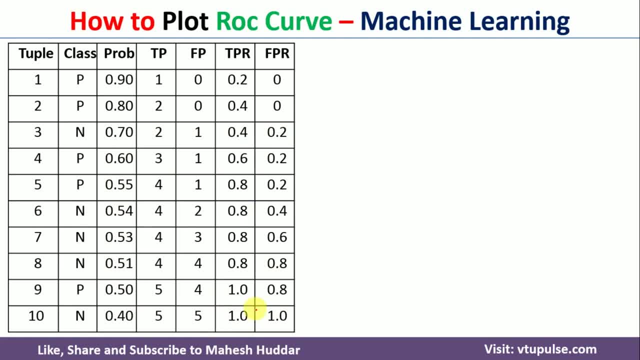 and FPR. for all these particular data points, we can easily draw this particular ROC curve. So ROC curve is drawn something like this: That is the ROC curve. So ROC curve is drawn, something like this: So ROC curve is drawn something like this: That is the ROC curve. So ROC curve is drawn. 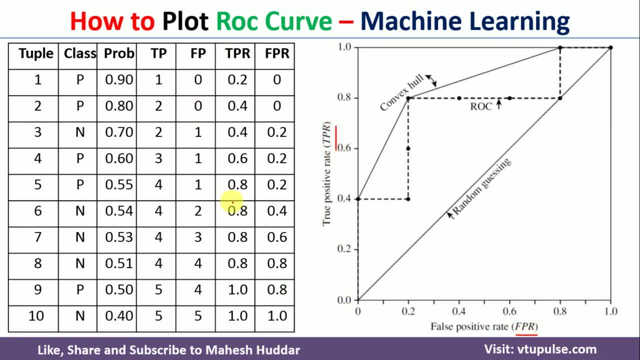 something like this: This is TPR against FPR. here We have already calculated TPR as well as FPR for all the thresholds, So I will start with this particular FPR that is 0 and associated TPR is 0.2.. So this is 0 and then 0.2 is this particular data point. 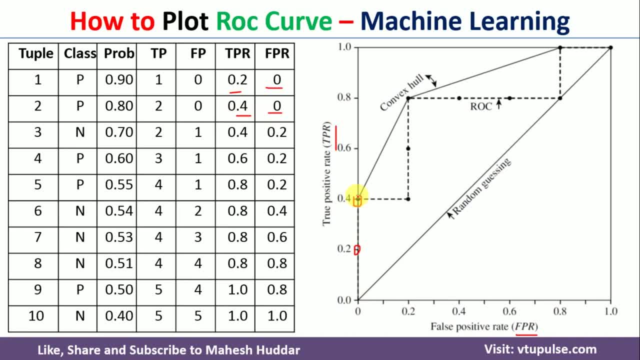 Second one is 0.4.. So again it is 0 and this one is 0.4.. The next one is 0.20.4.. So this is 0.2 and is 0.4.. The third data point is here. Next one is 0.2 and 0.6. it will come. 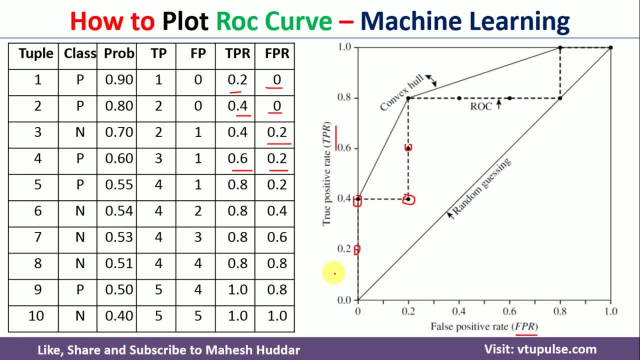 over here. we need to mark all these particular points and then we need to connect them. you will get final ROC curve over here. if you want to get the convex kind of well, you can use or you can connect these body things. you will get a final ROC curve here. so in this video i have discussed how can we. 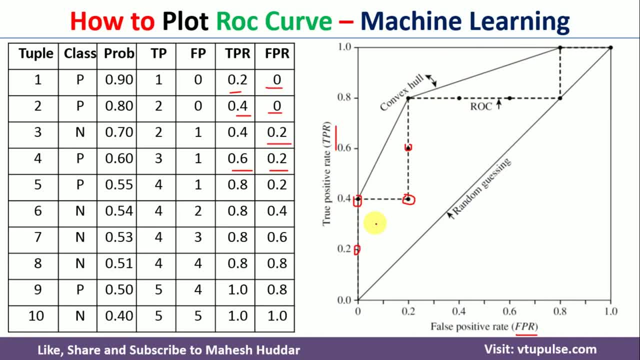 plot ROC curve for the given data points. i have already discussed one more example. the link for other example is given in the description below. if you like the video, do like and share with your friends. press the subscribe button for more videos. press the bell icon for regular updates.